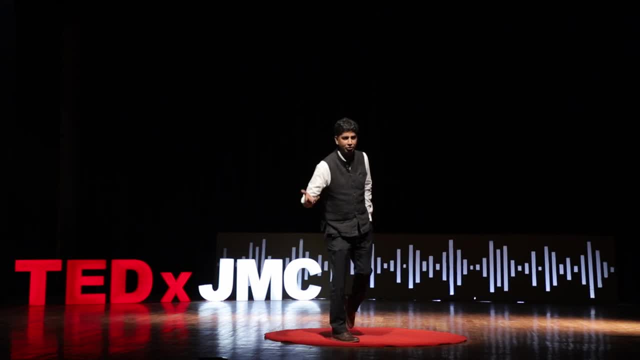 not drinkable. Which year did you read about a river pollution story in the newspaper? 2010,, 2011,, 2012,, 2013,. all these things that we talked about last 10 years, of course, several times. The name of the river can change, perhaps because we need newness in our stories. 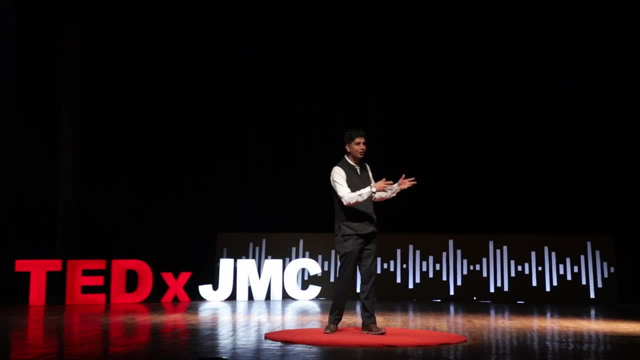 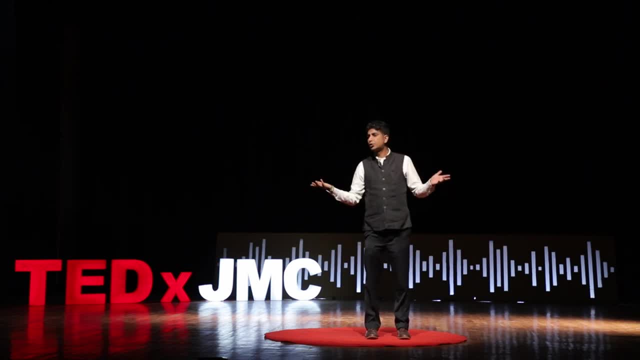 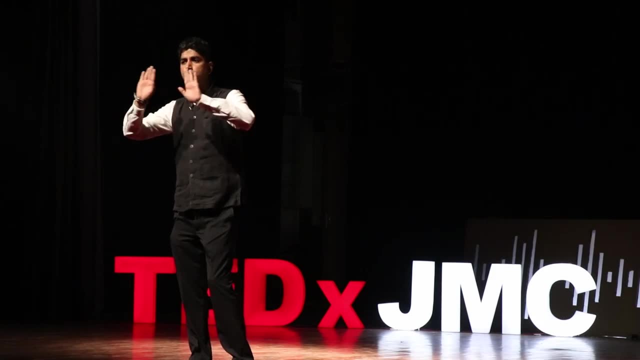 name for the river called Mithi, by the way, has been black for years together and we don't really know about it because it's all unspoken. Now, if you look at one thing, something that we spoke about- we've spoken about lakes, we've spoken about air, we've spoken about 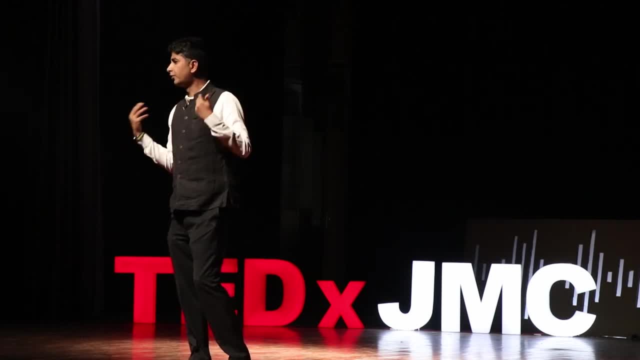 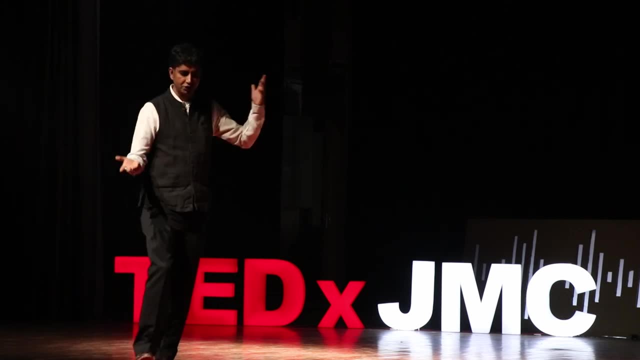 water. in that sense, You know every year what we do, the work that I do. I work with a foundation called Swetha. we work on environment. we work with young people, schools, colleges, people, trees, animals. We make an animal calendar. 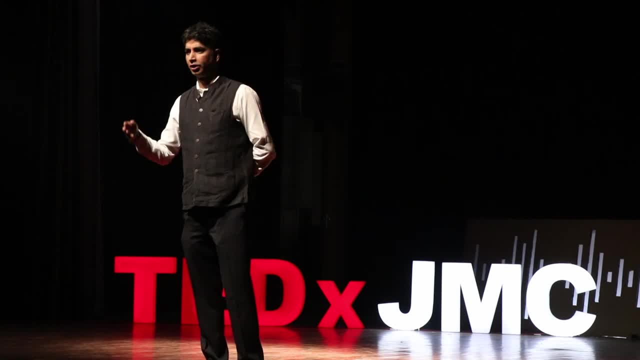 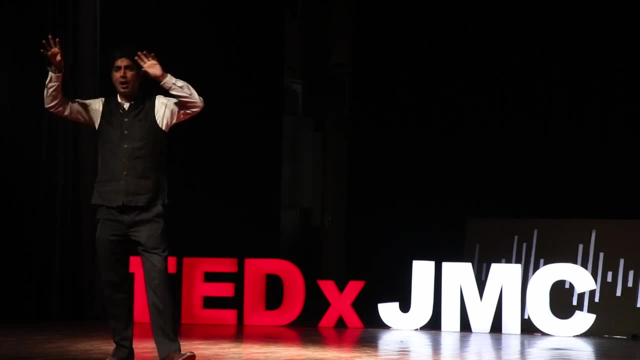 We make an animal calendar for ourselves to look at which month should we focus on what particular issue. So I made this very nice-looking, beautiful calendar which only had months, did not have dates, had Jan, Feb, March, April, May, June, July, August, September. 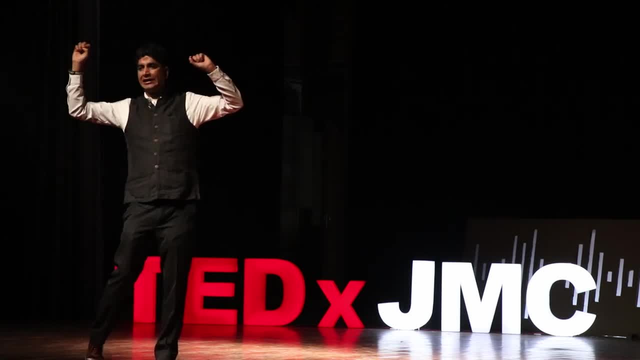 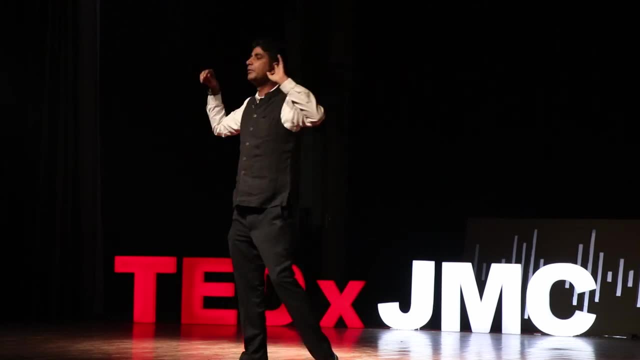 October, November, December, and on top it said 2016,. and I said fine, in the month of June, I'll actually be working on, say, forest fires. In October, I'll be working on air pollution. In December, I'll be working on Chennai floods. This is what the plan that 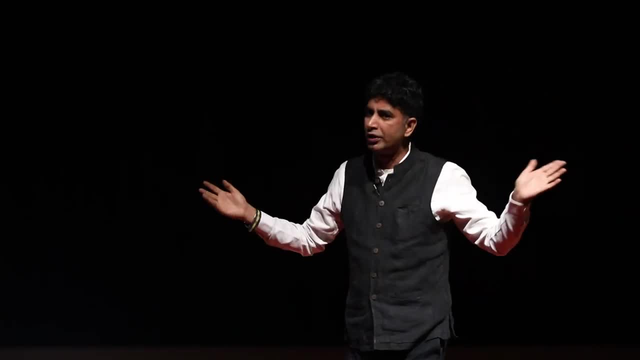 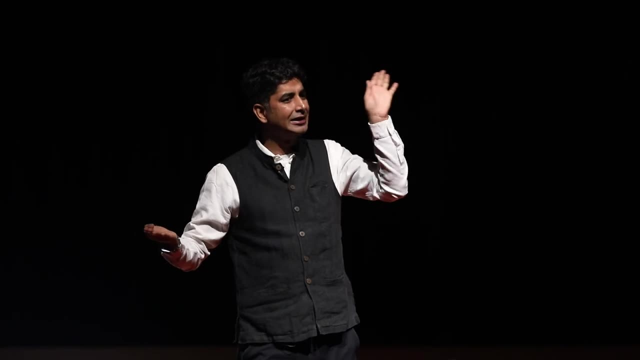 I made for 2016.. Now, December, khatam ho gaya. you know. 2016 was over. I was planning another one-year plan for 2017.. It was exactly the same calendar that used again in 2017 and in 2018.. And now, 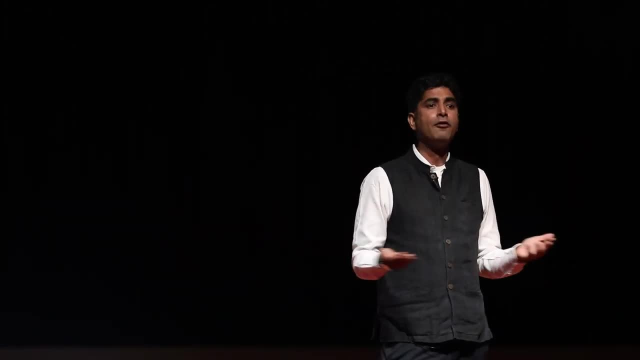 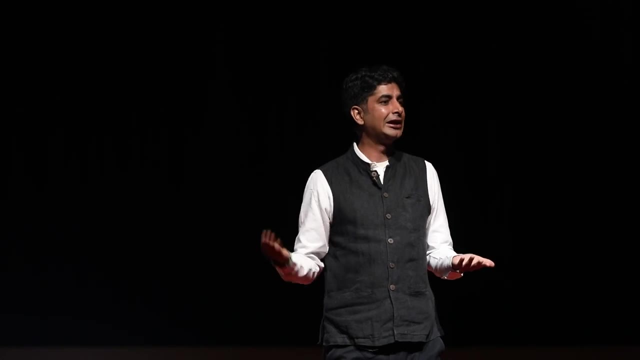 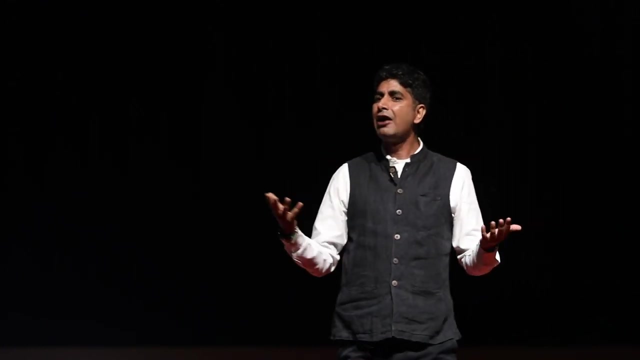 last month, when I set out to make a calendar for myself, for the organization, for 2019, my calendar looked the same. The same calendar that I made in 2016 still applies now, which fundamentally means that things have not changed Year after year. you and I wear a mask. read a story about a burning, frothing fuming. 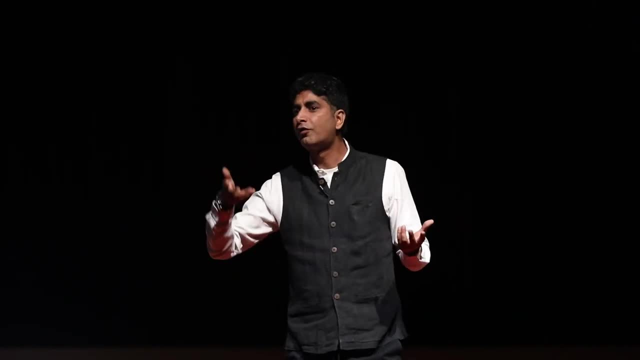 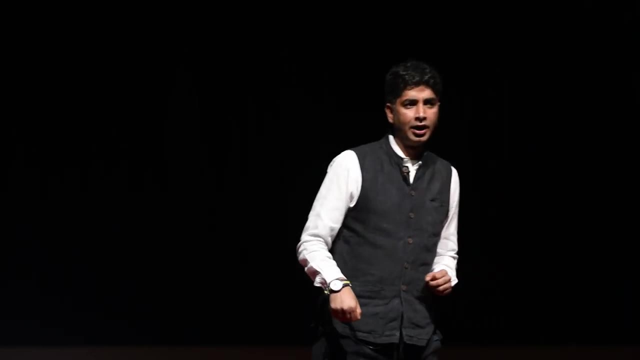 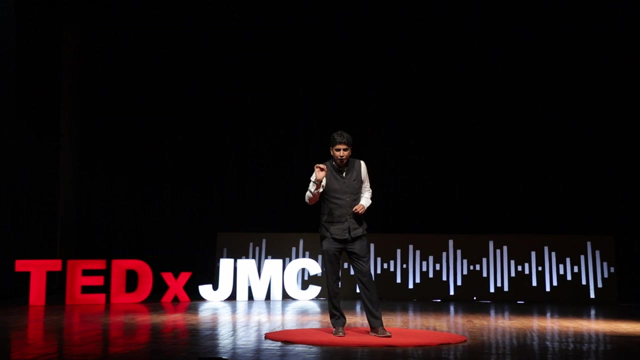 lake, or we all read about many of these other environmental issues- like it could be of a huge forest that perhaps is disappearing in Mumbai or could be in any other part of Gurgaon. These are all spoken, but foolish people like us, we do not hear it, We do not. 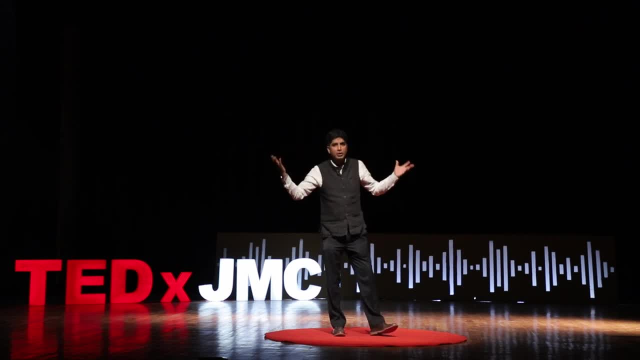 think it's unspoken, It's a vow of knowledge that someone needs to come on a TEDx talk and tell you about these issues when it's almost on your front page on your face. Forget about being on your front page of a newspaper. It's on your face as a mask, as your water. 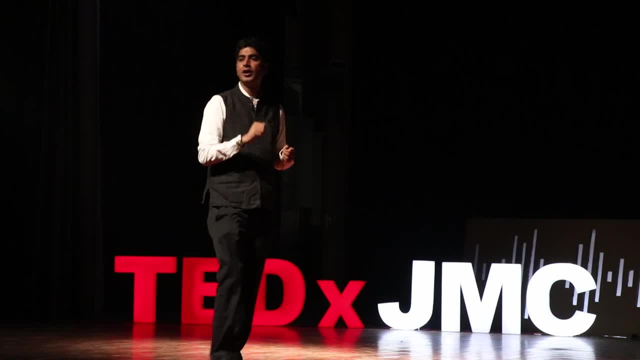 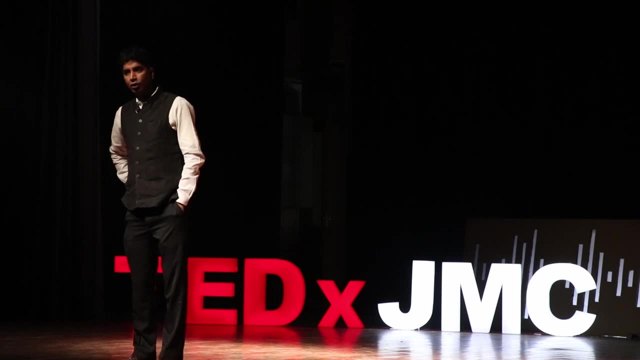 as your real visual of a froth. in that sense. Now, some of these issues that we have talked about right now, I need to explain a few things to you: Bangaluru, Bangalore- it's easier to say Bombay than Mumbai, so Bangalore in. 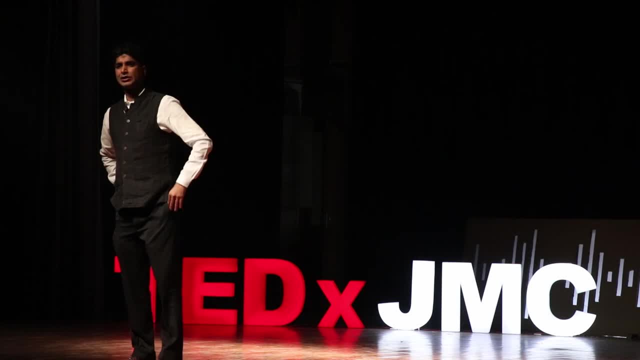 that sense. you know, had many, many lakes. The city was actually planned in 1600, the way they had planned the entire thing there was a natural way to preserve water. Almost 300 lakes is what Bangalore had and by 1970, almost all the lakes have either. 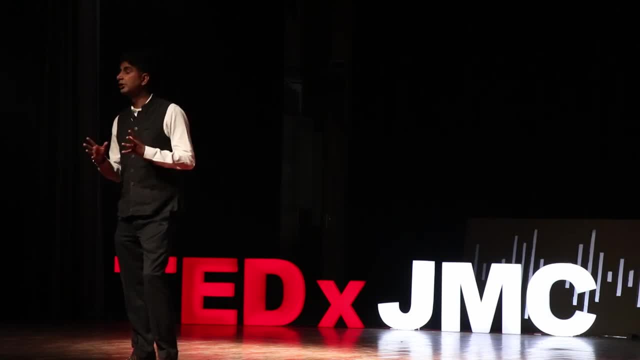 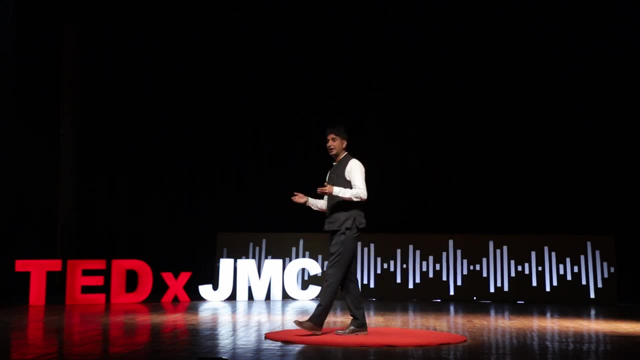 disappeared or have actually become extremely, extremely polluted. 1,200 million liters of wastewater- municipal wastewater- enters these lakes every day. That's the amount of waste that Bangalore actually creates. We're not even- we're only talking about water right now. imagine this so-called Silicon. 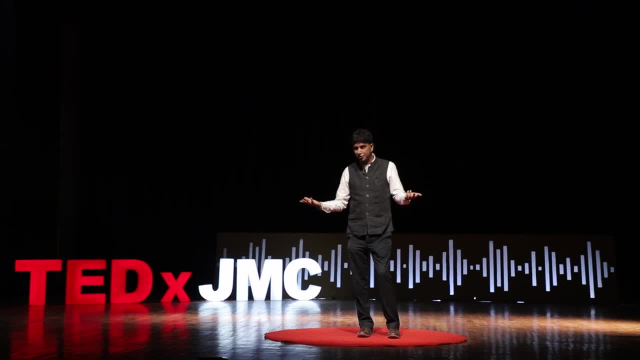 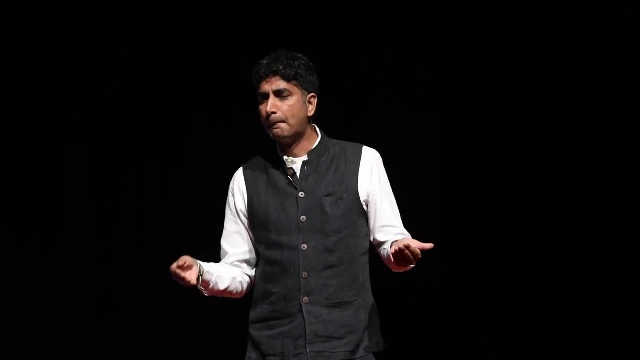 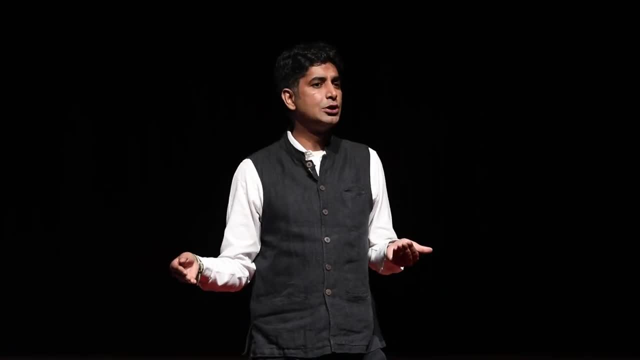 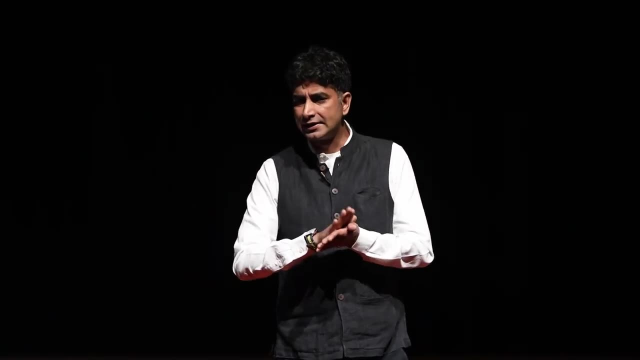 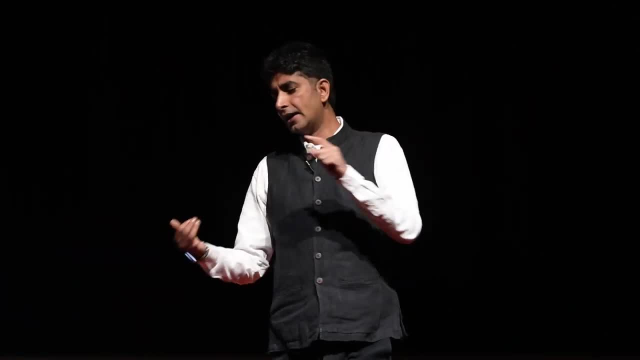 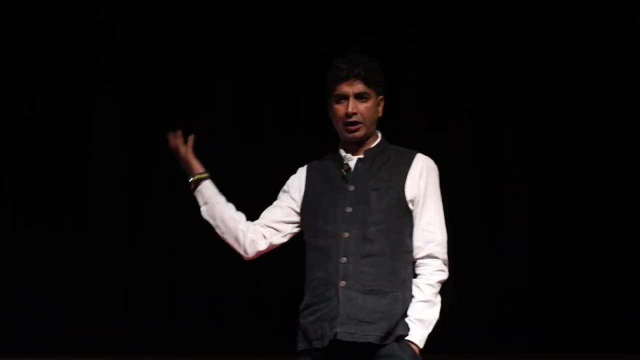 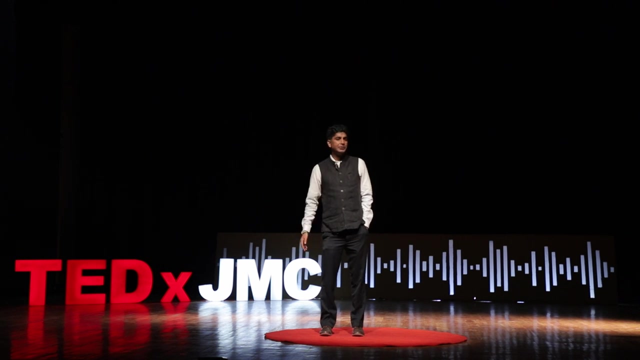 there's almost like a mountain of froth almost every second day. Second story that I'm going to share with you is about another modern business capital, one of the richest cities that we actually have in our country, called Gurgaon. Gurgaon, you know, there's hardly any water. the trees are disappearing. Just last week, 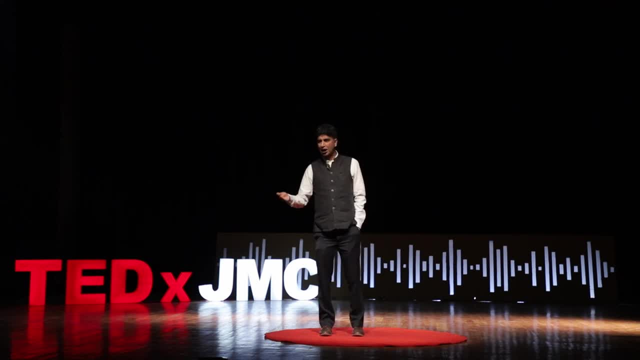 it was actually rated. it got an award, a very fancy Achhedin award, for Gurgaon to be the most polluted city in the world. right, And when we are actually leading and hearing about such amazing statistics called the most powerful polluted city of the world, what? 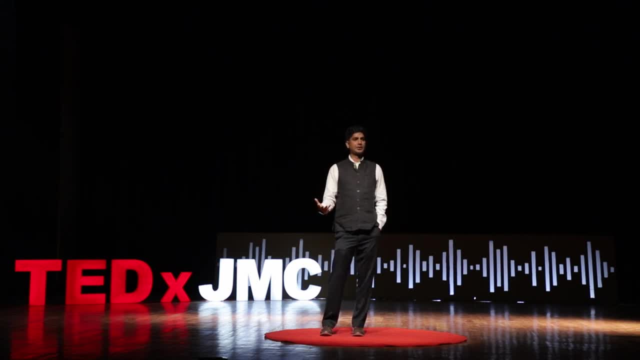 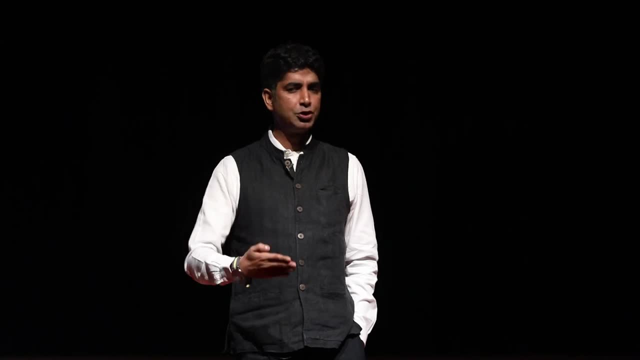 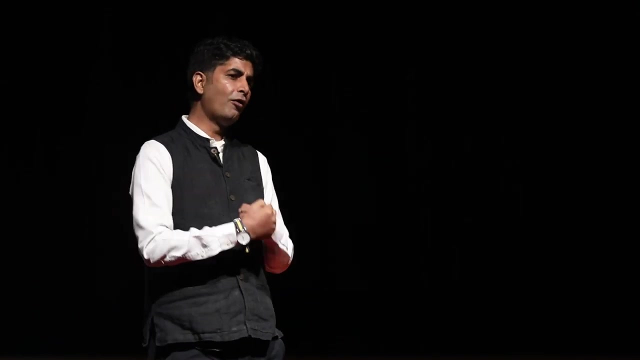 does the government do? Citizens of our country, citizens of Gurgaon, had set up a forest called Aravali Biodiversity Park, planted almost a lakh and 25,000 trees over years together through citizen action. but government says, oh well, it takes so much time for citizens. 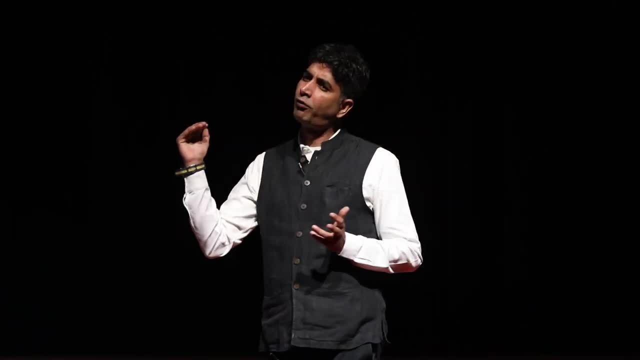 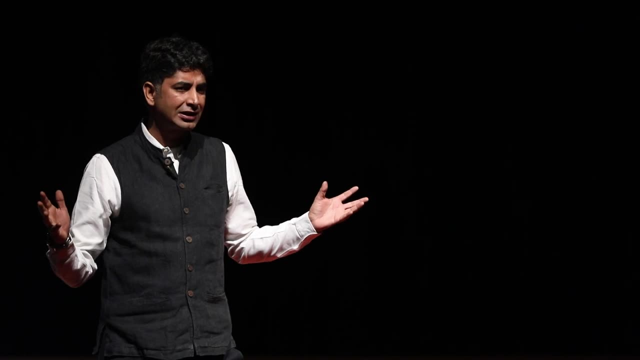 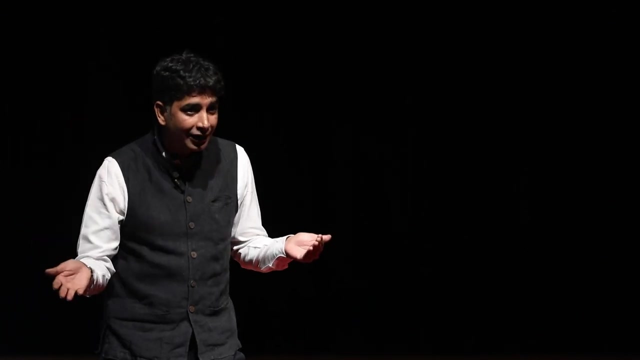 of Delhi and Gurgaon to reach Manesar. cars need to move faster and faster and therefore let's build a six-lane highway through this Entire forest. that was not created by the government. that was created by the citizens over their own sweat and love and work. we want a highway. We want a fancy highway Did. 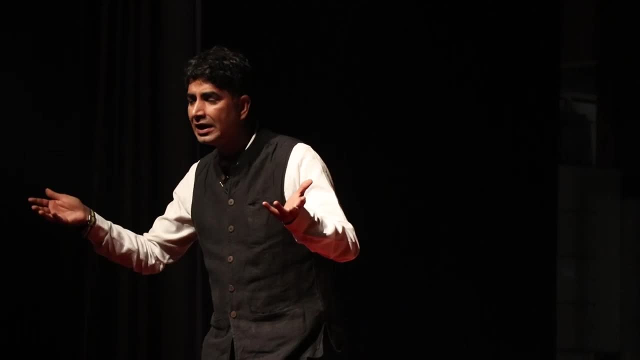 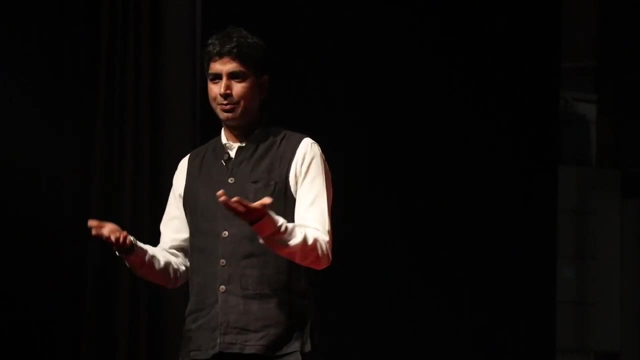 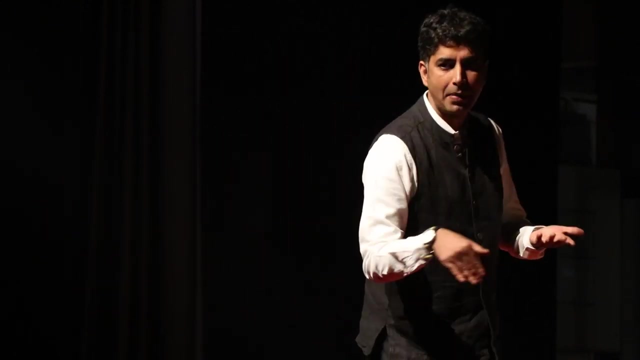 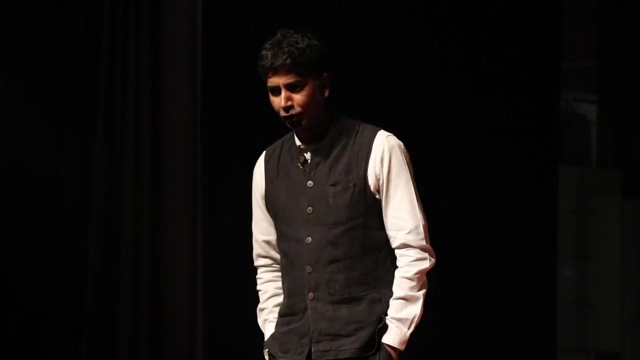 people speak. Some people did. Many of you us did not speak at all, because Gurgaon is a fancy city. cyber hub is so amazing. every restaurant is there and you know, the nightlife is With the 福 길젠골. 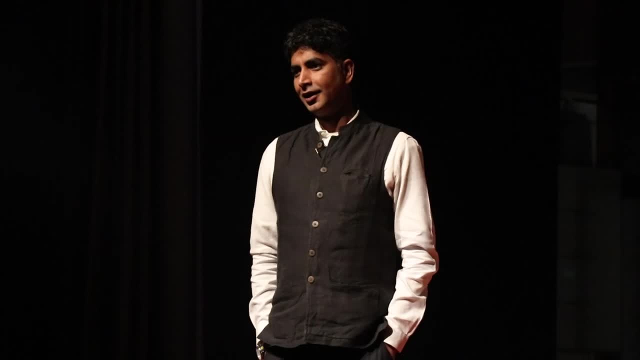 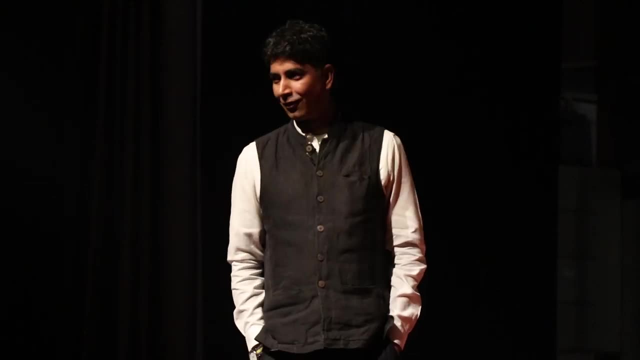 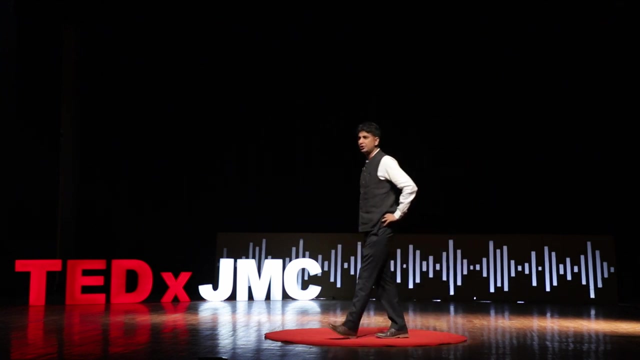 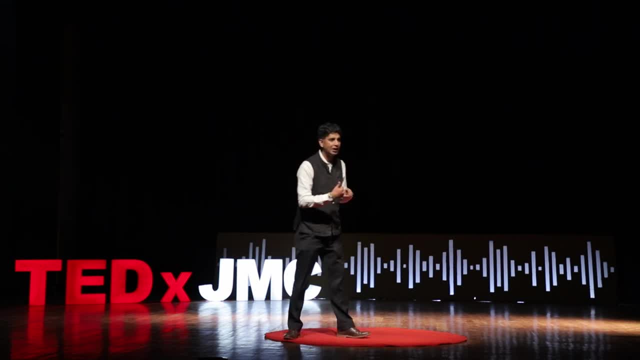 in Sarojini Nagar area, in Netaji Nagar area, in Nairoji Nagar area. Many of us spoke about it for months together, but citizens of Delhi perhaps want more malls. Do you need more malls in Delhi or do you need fresh air? 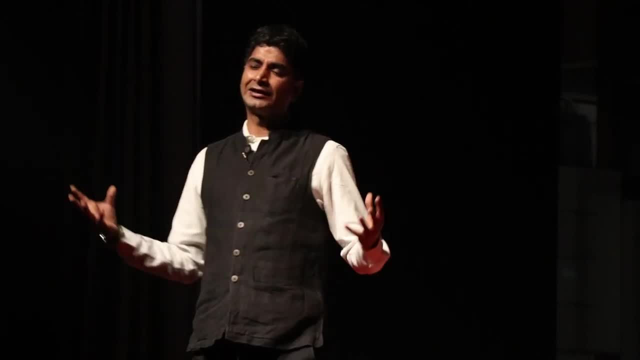 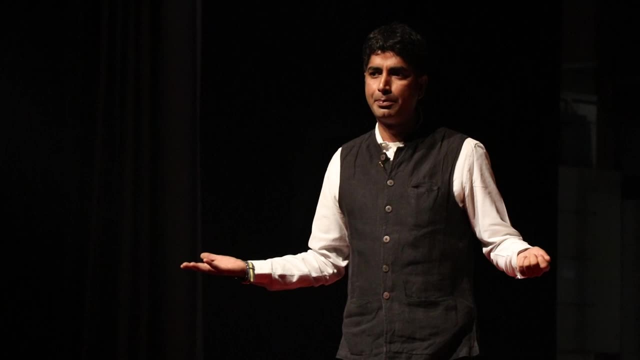 Do you actually need more days to live? Do you think it's fashionable to really wear a mask and walk into your classroom? Is there a fashion? I'm sure eventually there will be a brand that will say: oh well, you know, this one looks cooler. 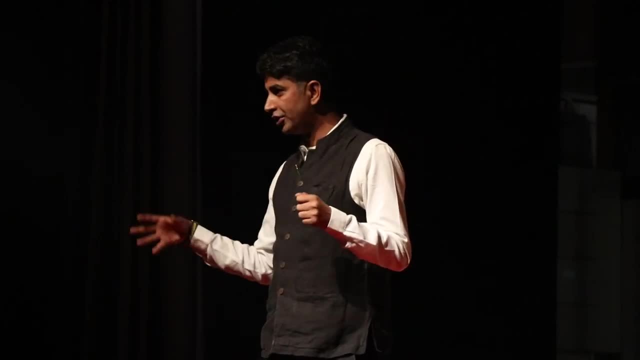 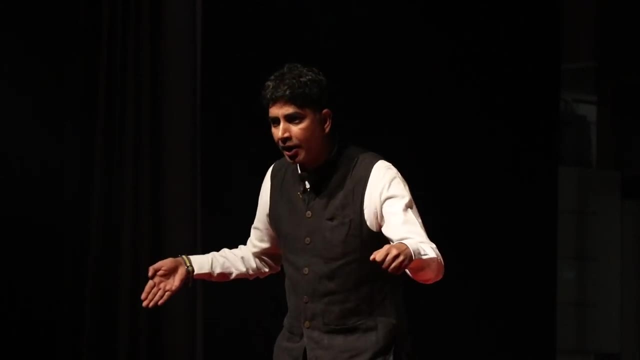 This mask is cooler than the other, or this one is in vogue, or the other, I'm sure, Because you don't have a choice. You will not have a choice but to wear a mask to your potty room. That's the reality that we all are signing up for. 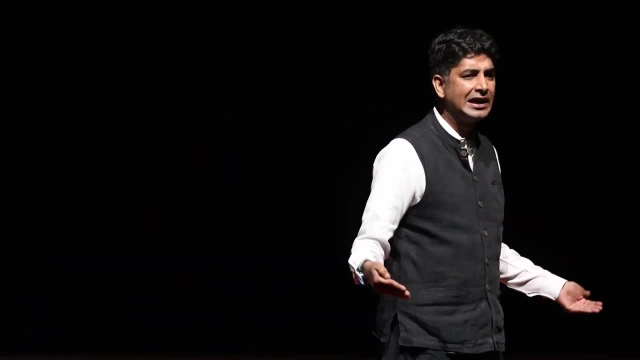 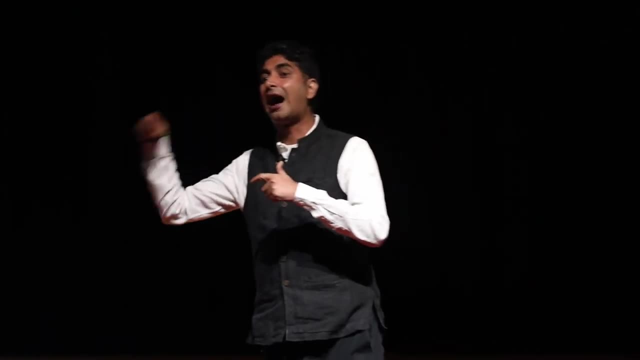 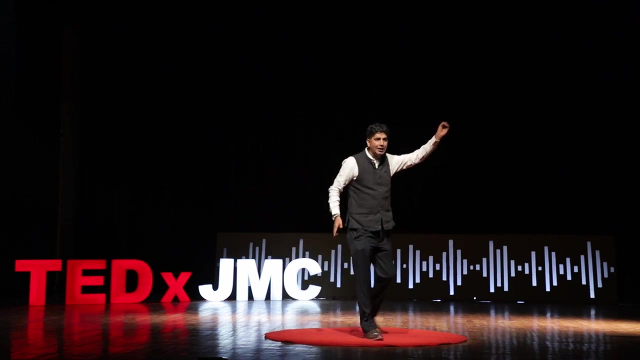 But why are we all not speaking up about these things that are there staring at our face? This is not somebody else's problem. This is not that I've dug out and found out from Dantiwala or from villages of, say, Tamil Nadu. 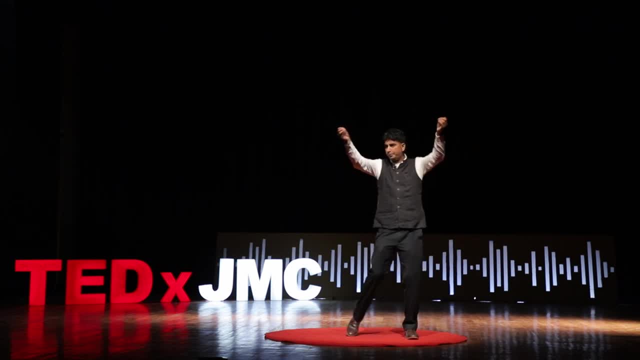 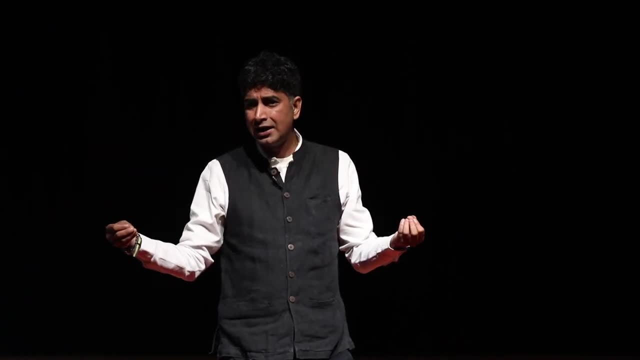 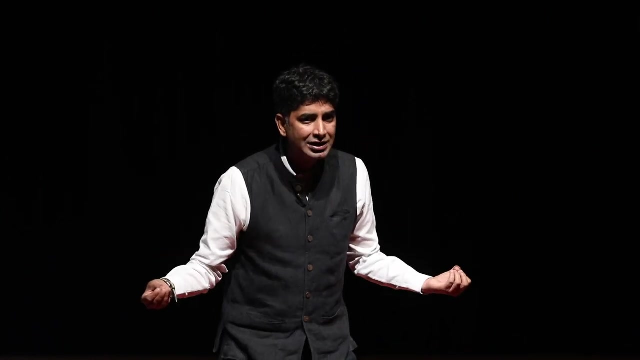 These are stories of the biggest. These are the big cities of our country. Groundwater: The government report says that by 2030, almost 21 major cities of our country will not have groundwater at all. Delhi is going to run out of water in a few years. 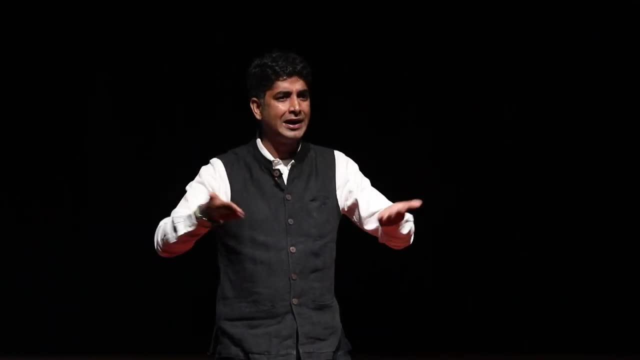 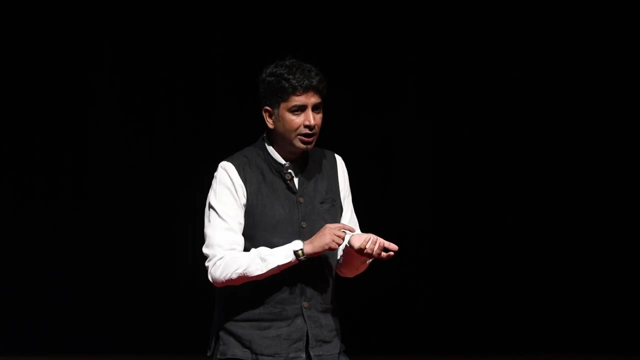 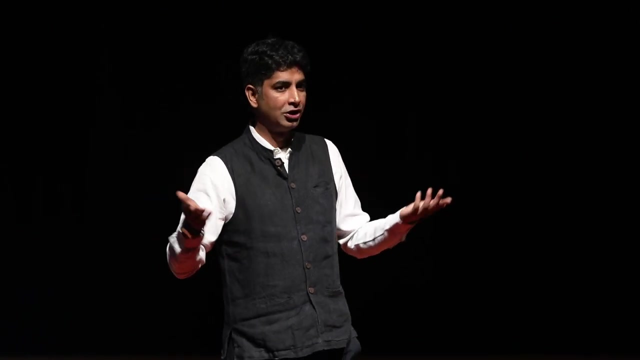 These things that are actually spoken about already is in public domain And if it does not solicit reaction, response behavior, some kind of a Tuck-tuck to you, To Woleka Kappa, it's better, That is, that it's not spoken. 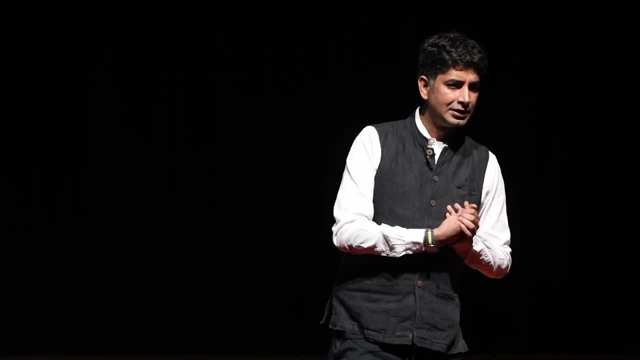 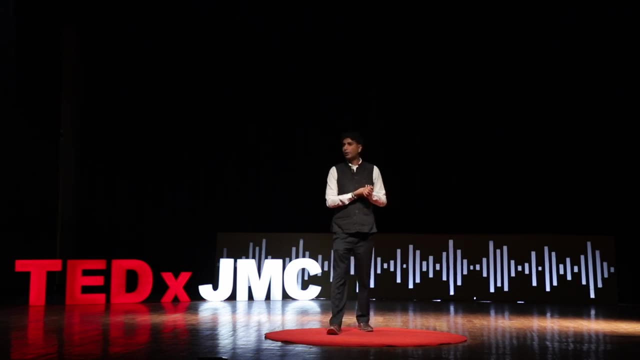 It remains unspoken. I will end with sharing with you something. when people spoke, There's a there's 40 percent of our India's copper comes from a factory called Sterlite. You know, in 90,, 90,, 90 to, there was a factory that was to be set up in in Ratnagiri in Maharashtra. 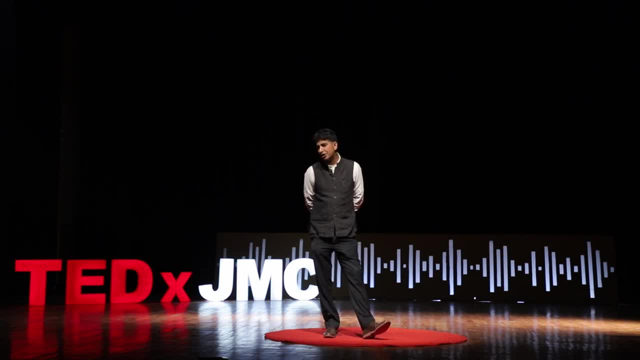 It. The people there protested. They said they do not want a factory in their back backyard. They protested, Ratnagiri had to move the entire factory somewhere And suddenly Tamil Nadu said: oh well, come set up this factory in my backyard, violating every environmental norms. 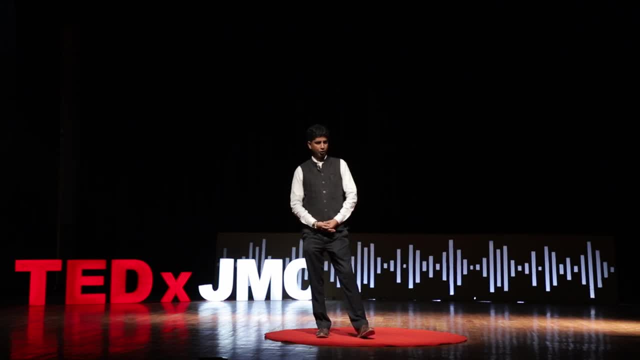 Sterlite was actually set up in Tuticorin in Tamil Nadu in 94. Since then, several times, several cases, every rule have been violated. They've been challenged, shut down by the Supreme Court, by the High Court, by the pollution control boards, because people there, the poor people there, the farmers and the citizens actually, you know, every week there were cases of breathlessness and sometimes cancer. 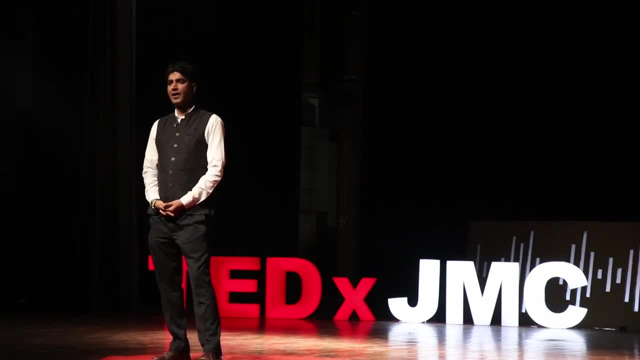 Many people just last year. it was March, in fact. last year they said enough is enough. They had actually protested earlier as well. They got together and they were protesting against this factory that was killing them. It wasn't about anything else. 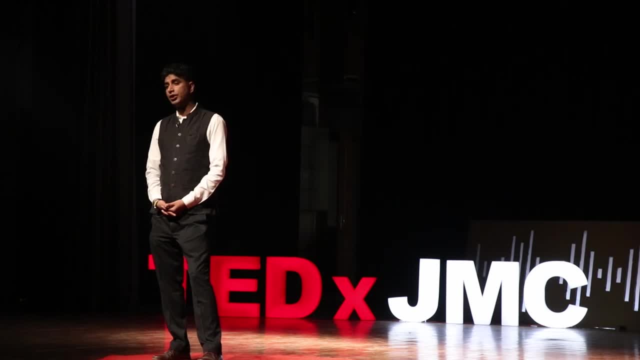 It was actually killing them And they started protesting on the streets of Tuticorin. What happened? There were 13 people who were murdered by the police in broad daylight for speaking up- And they were speaking up for clean air, clean water and a right to live. 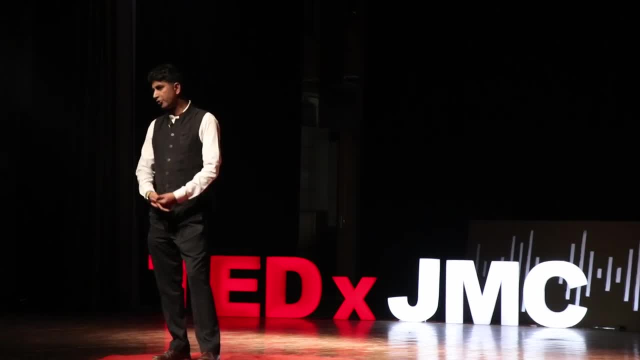 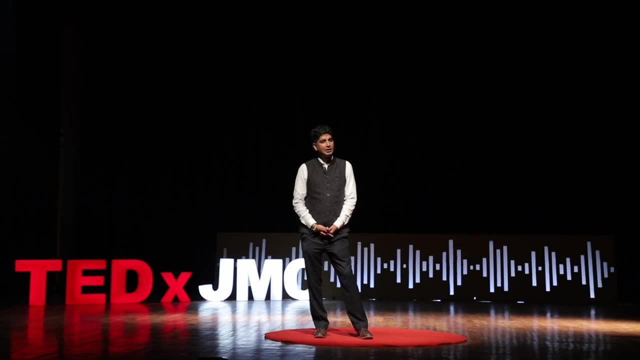 Now two things here about everything that I've spoken right now. Two things. One: You know we cannot leave the business of speaking to the poorest of the poor, Poorest of the poor, do not have the agency We have to. 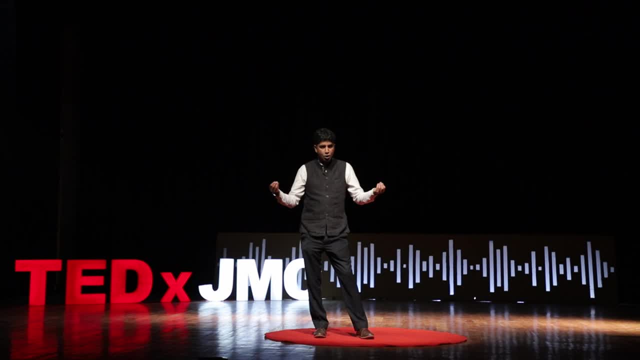 People like yourself and myself and all of us who have more agency, who speak English, who eat burger, who actually have better lifestyle, can afford to stand up. We need to speak up for ourselves and also for the poorest of the poor. We need to speak up for the poorest and the poorest and the marginalized of our country. 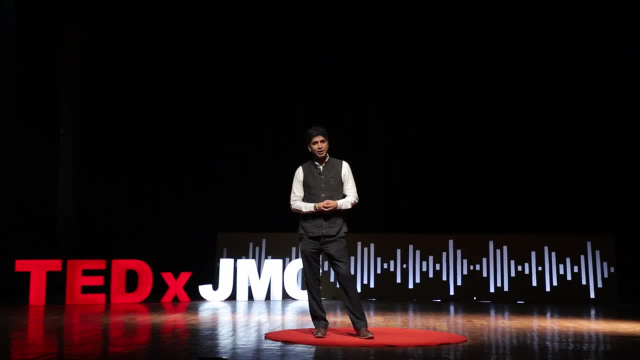 Because if we do not speak up, there's no planet. You know, you can imagine that perhaps you can buy a lot of these things, buy fresh air, but our air doesn't come from an air purifier- It will actually, it comes from trees. 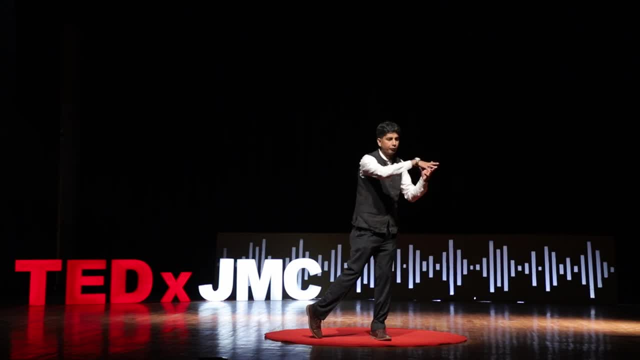 Your water does not come from a water purifier or an aqua guard. It still comes from your rivers and your underground water. You need to go. you know education. Our education needs to be applied at the right place And we all need to speak up and hear up and do things around us.